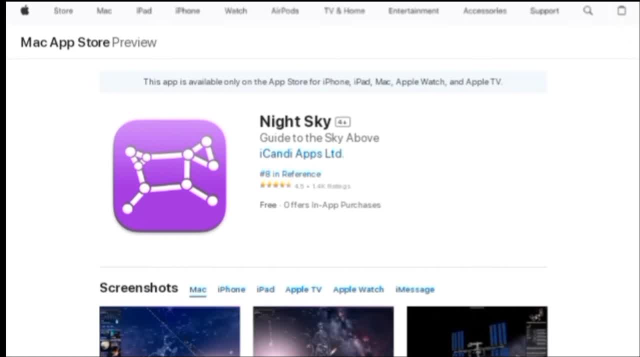 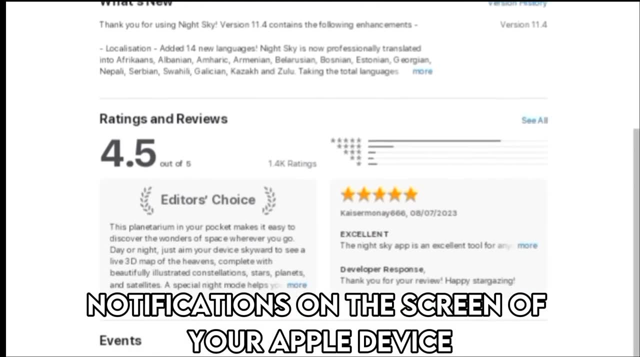 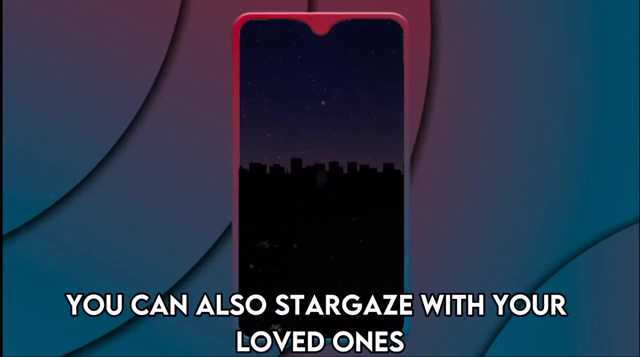 NightSky – Best for Apple Users. This app enables you to tour the sky and receive sky notifications on the screen of your Apple device, including an iPhone, Mac, iPad, Apple TV or Apple Watch. You can also stargaze with your loved ones even when you're apart. 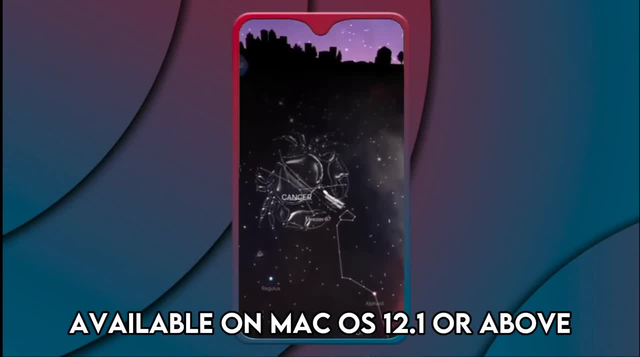 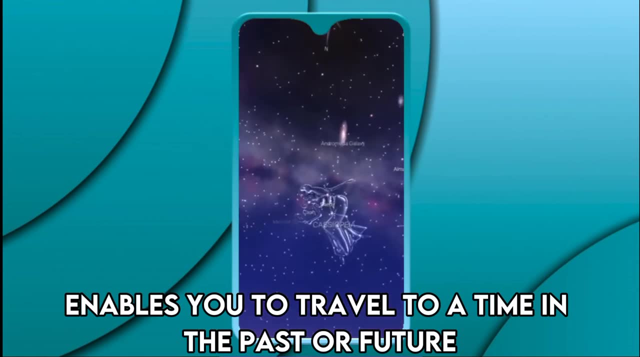 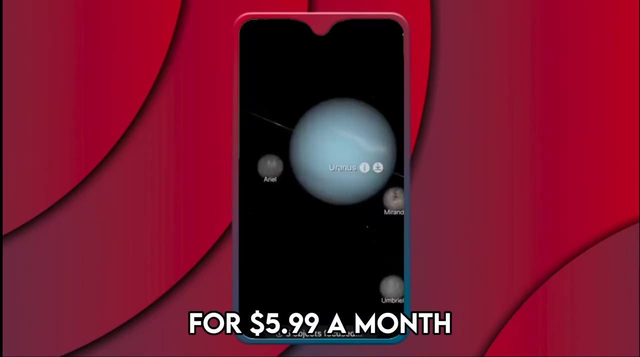 a new feature that's currently available on macOS 12.1 or above. NightSky has a space travel feature that enables you to travel to a time in the past or future. then timestamp it for quick access anytime you want, For $5.99 a month or $39.99,. 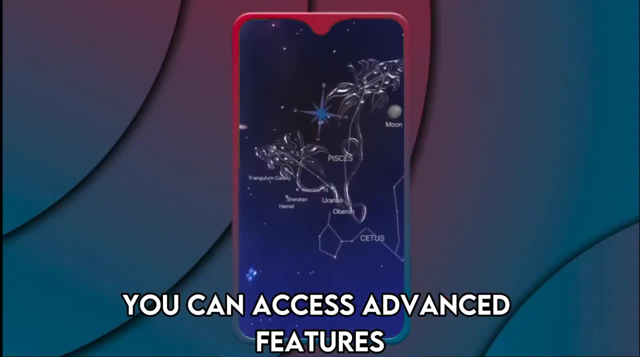 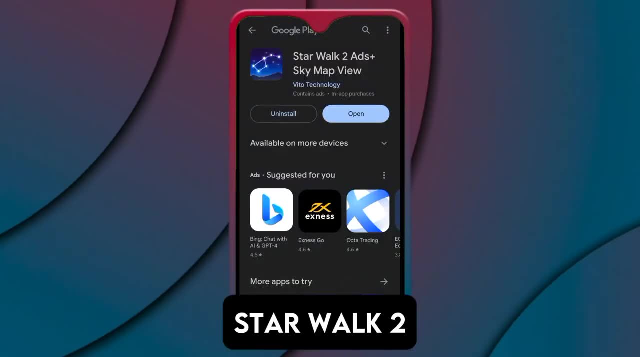 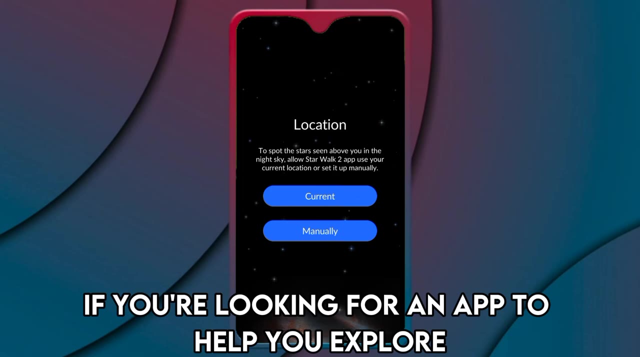 you can access advanced features designed to make your stargazing experience unique and memorable. StarWalk 2 adds plus SkyMap View – Best Astronomy Guide app If you're looking for an app to help you explore and learn about different stars, constellations, satellites, planets. 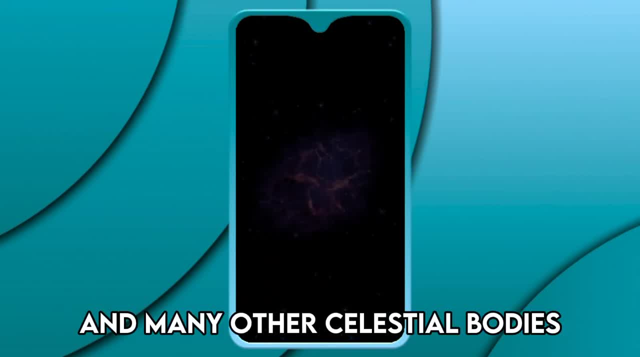 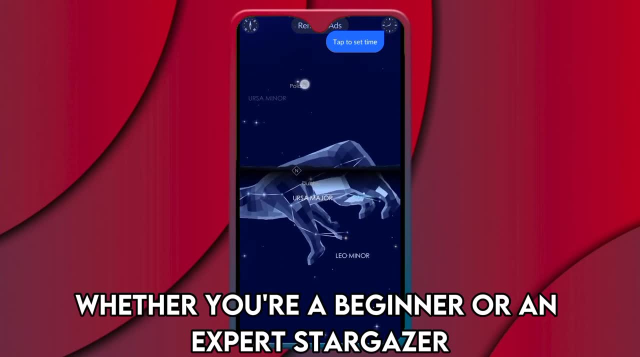 deep space objects and many other celestial bodies, then StarWalk 2 is a great option for you, Whether you're a beginner or an expert stargazer. you simply need to point your device to the sky and access a real-time view of the SkyMap. 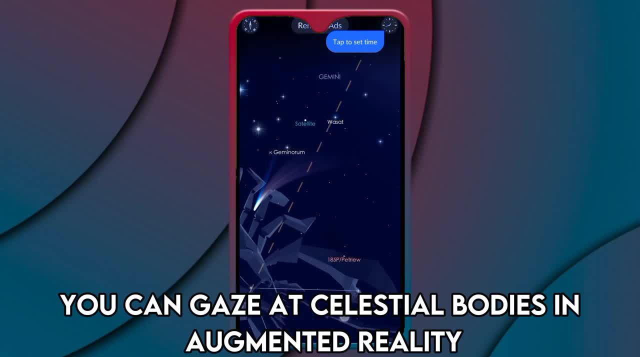 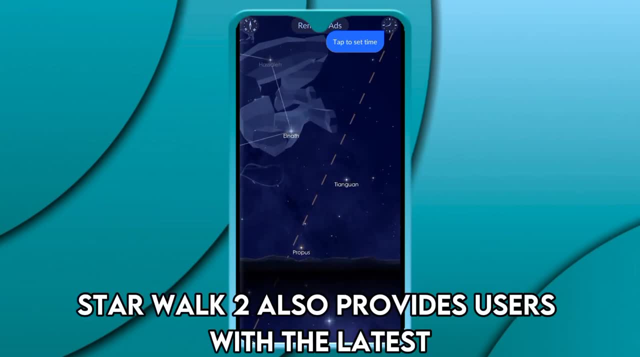 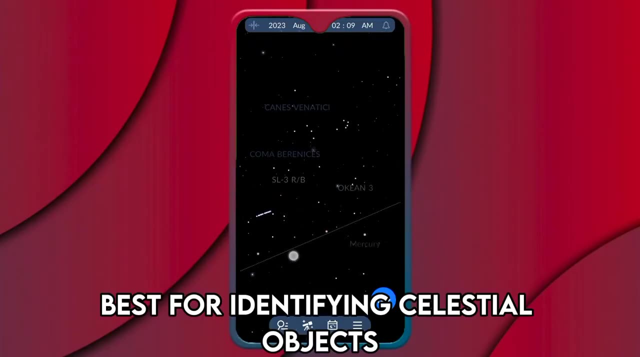 You can gaze at celestial bodies in augmented reality, making stars and constellations seem closer than they are. StarWalk 2 also provides users with the latest space news and astronomy events Sky to Night – Best for Identifying Celestial Objects Brought to us by the developers of StarWalk 2,. 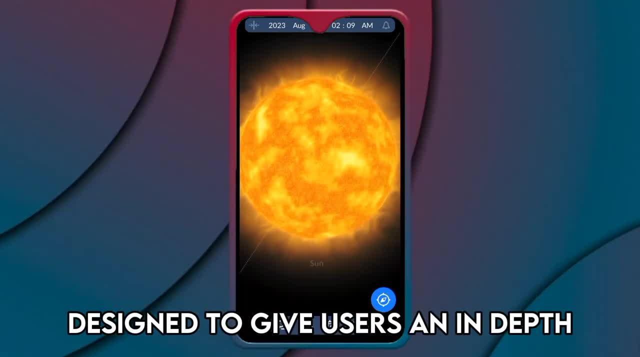 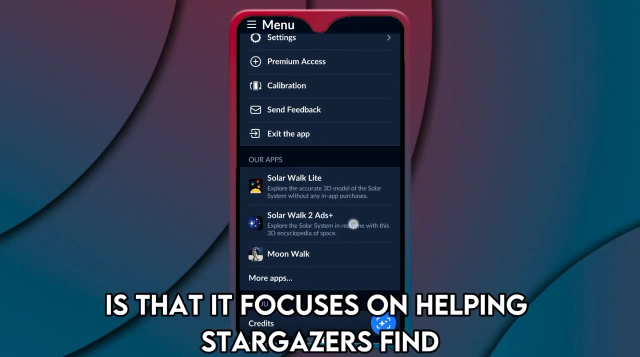 Sky to Night is another app designed to give users an in-depth real-time view of the sky. The main difference that sets it apart from StarWalk 2 is that it focuses on helping stargazers find and identify specific objects in the sky. 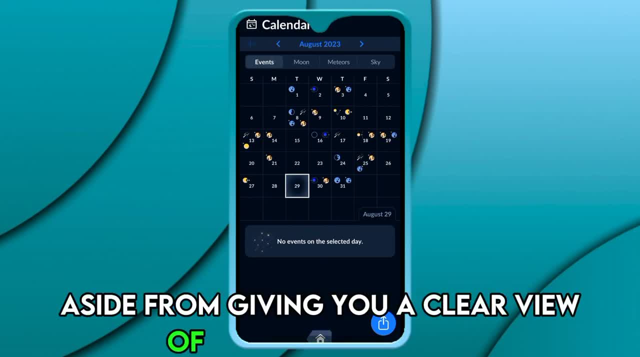 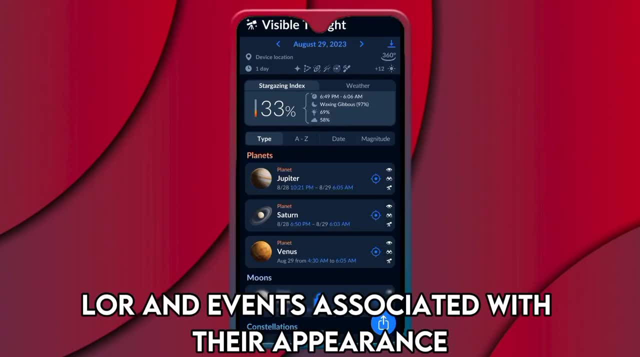 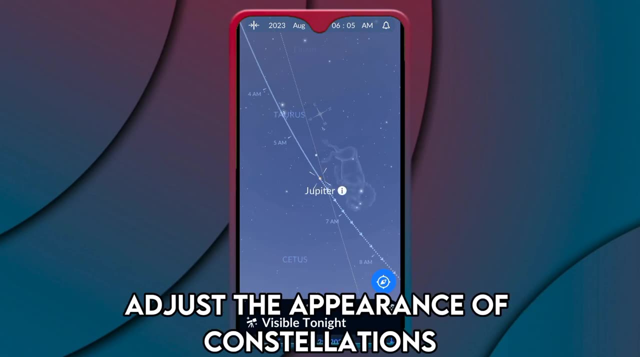 Aside from giving you a clear view of stars and planets, it also provides you with their history, lore and events associated with their appearance. Like with other top stargazing apps, you can view the position of stars at different time periods, adjust the appearance of constellations.